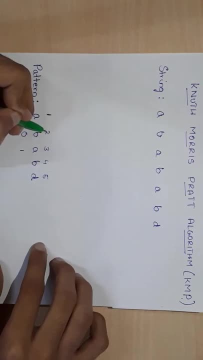 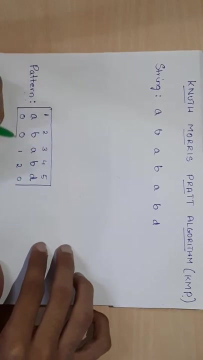 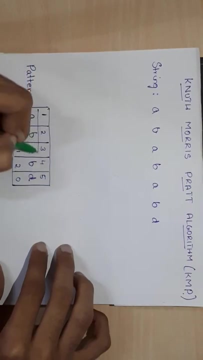 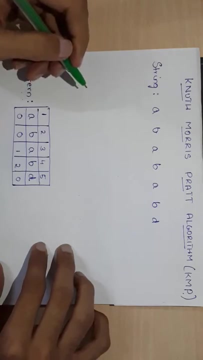 And for this b, another repetition. So this index number is going to be put over here. For d, there is no repetition, so 0.. This is the particular pie table. Okay, After creating the pie table, we need to take two new variables, that is, i and j. 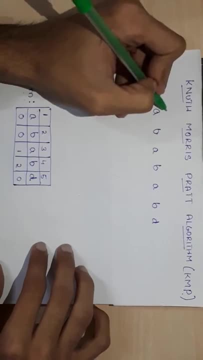 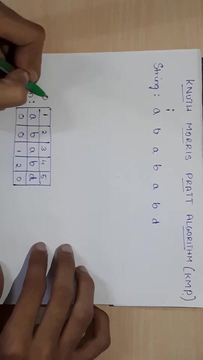 For the i, we are going to insert it on the first alphabet over here. And for j, we are going to put: before adding the j to the pattern, we are going to add a 0th index over here And the jth value will be over here. 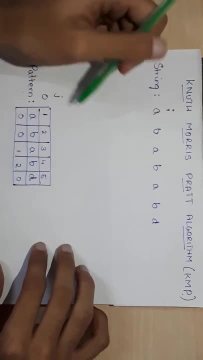 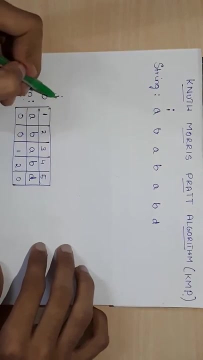 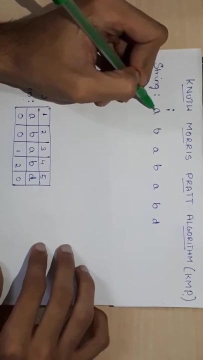 So how does KMP work exactly? So the j plus 1's term must be equal to the i's term. Remember, the i's value will be incremented and the j's value will also be incremented. So let's compare: j plus 1's term is a and i's term is also a. 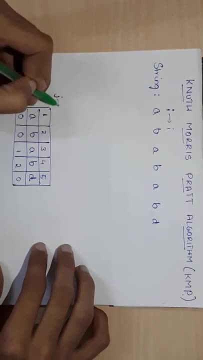 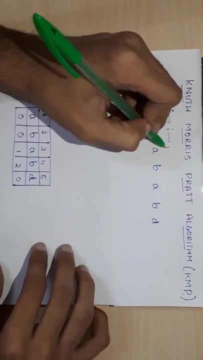 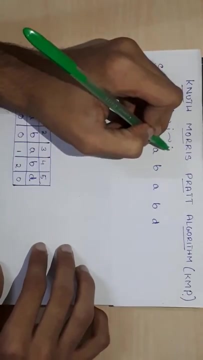 So i gets incremented. j also gets incremented. Now j plus 1's term is b and i's term is also b, So i gets incremented. j also gets incremented. Now j plus 1's term is a and i's term is also a. 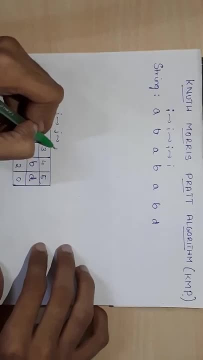 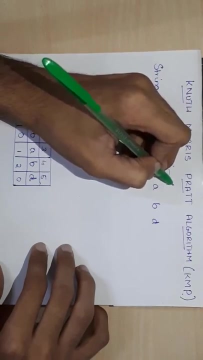 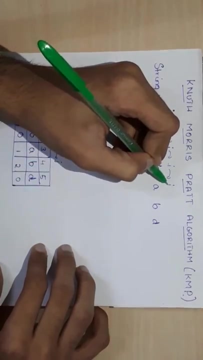 So i gets incremented. j also gets incremented. Now j plus 1's term is b and i's term is also b, So i gets incremented. j also gets incremented. Now j plus 1's term is d and i's term is a. 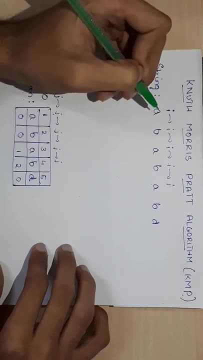 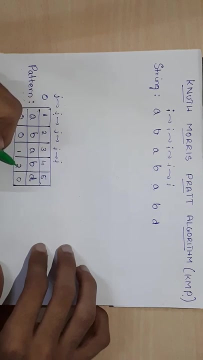 We are getting a mismatch over here. So whenever we get a mismatch, the j's value will be backtracked to its respective index quotient, That is in this column. the particular number we are given here is 2.. So the j's value will be shifted over here. 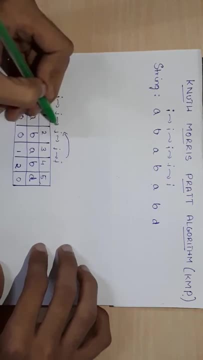 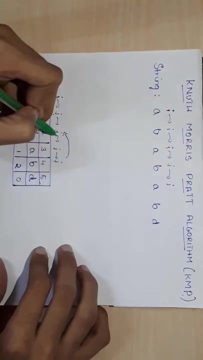 So this j plus 1's term is a and i's value is also a, So the i gets shifted over here. I mean the j's value gets shifted over here and the i's term gets incremented by 1.. Now the j plus 1's term is b and i's term is also b.